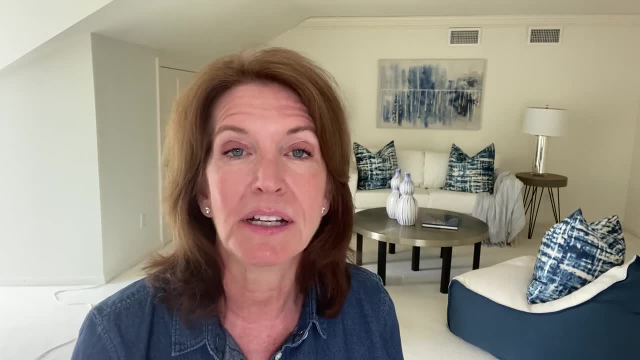 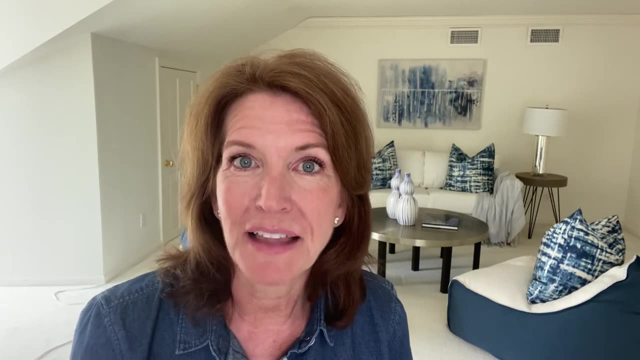 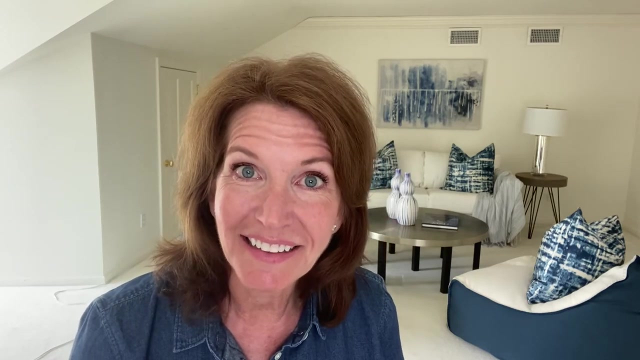 Over the years, though, and the months and then the years, my son started to be able to crack the egg in the batter, pour the flour into the mix and eventually pour the batter on the griddle and then flip the pancakes. It wasn't long before he was able to get up in the morning on the 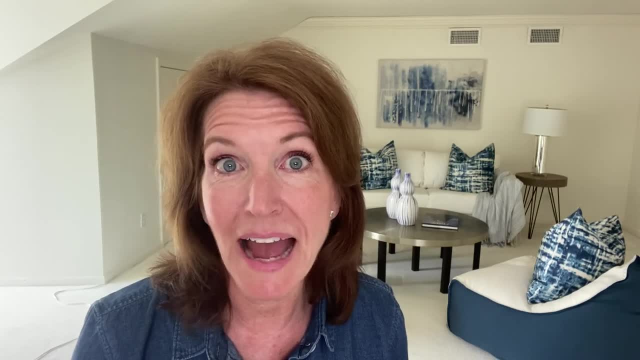 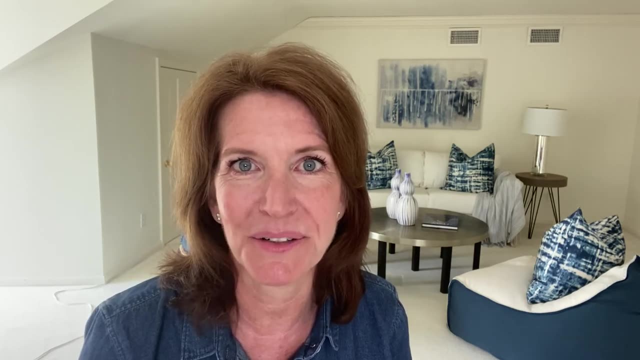 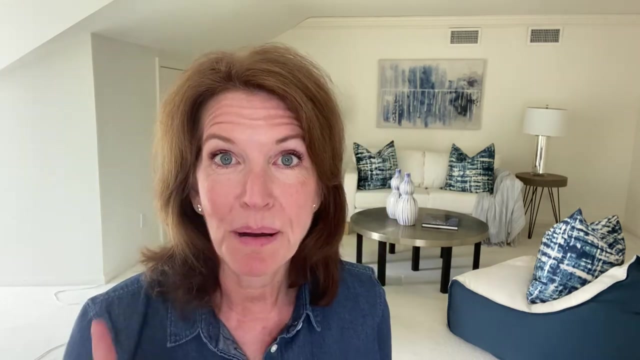 weekends and make the batter himself and make the family our pancakes. So we have to start somewhere, and toddlerhood is the perfect time to do it. So I want to give you five ideas so that you can get started with the toddler in your life. But before we go through those five different ways, 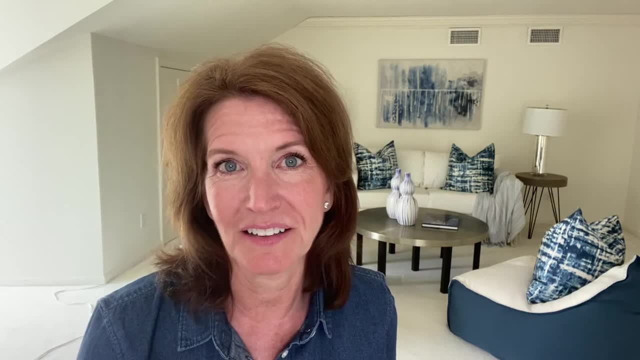 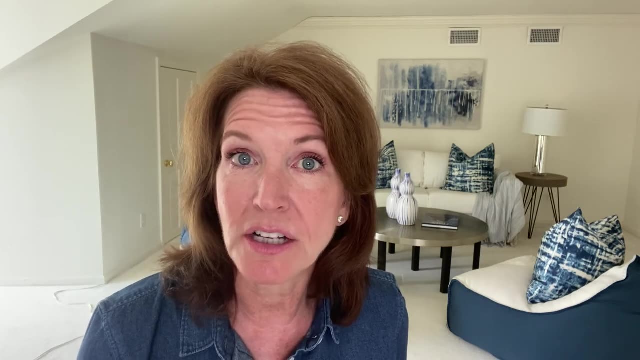 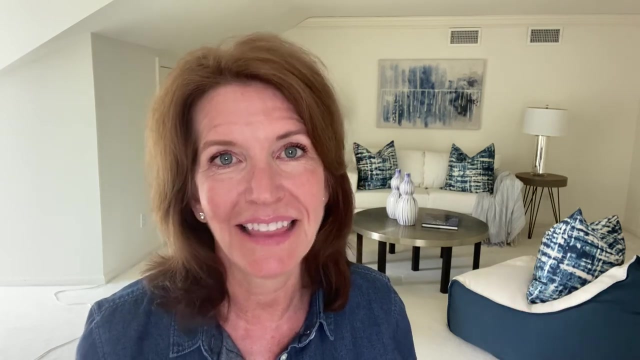 I do want to say that there's a huge benefit to toddlers to get started with cooking. Number one: it really feeds into their desire to be independent. autonomous Toddlers like to do it themselves. In fact, they'll say, no, me do it. That is that independent streak that they have, which is developmentally normal. 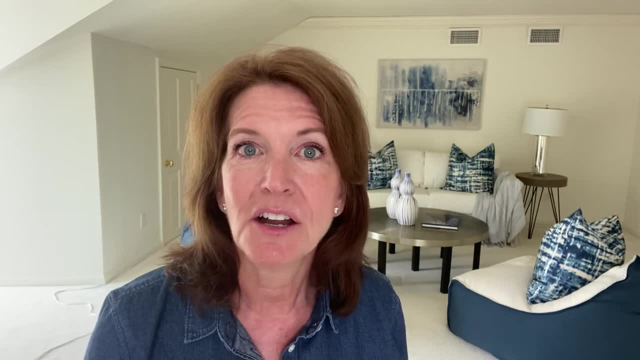 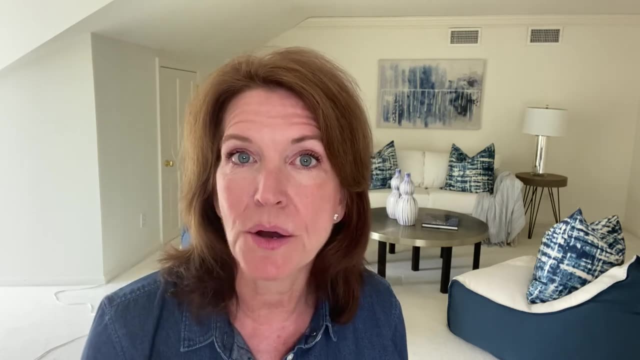 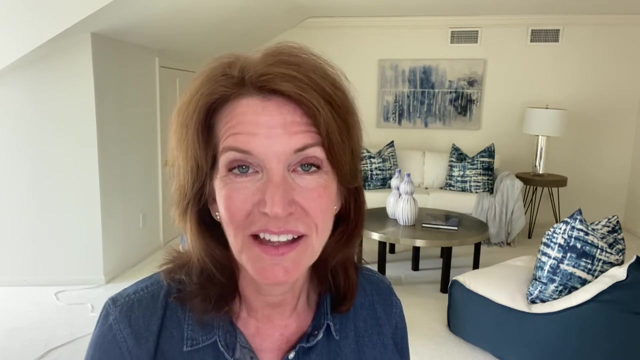 for them. So allowing them to get involved in the kitchen really feeds into that desire to be independent and that developmental milestone. We also know that toddlers who are involved in cooking tend to eat the things that they are involved with. So for those of you who are, 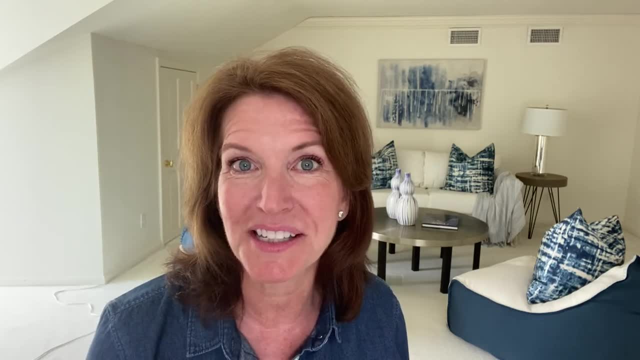 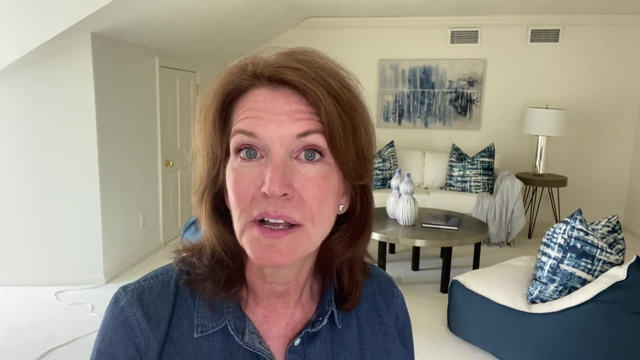 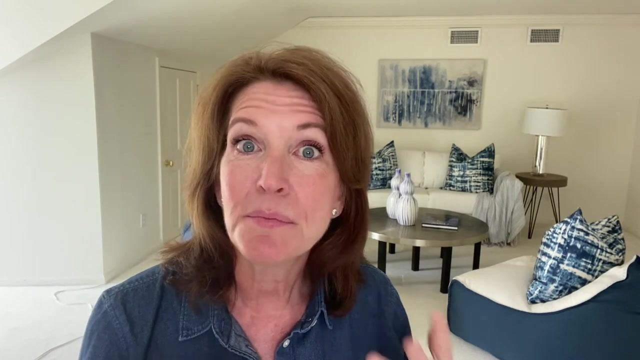 out there who have picky eaters that won't eat vegetables. get your toddler in the kitchen tearing lettuce or sorting different vegetables or stacking baby carrots, whatever. The more hands-on they are with food, the more likely they are to taste and eat those foods And getting kids in. 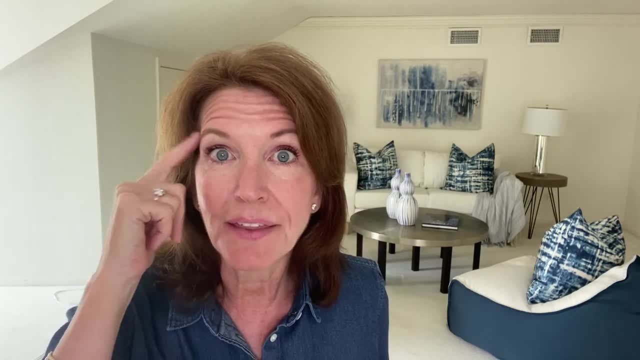 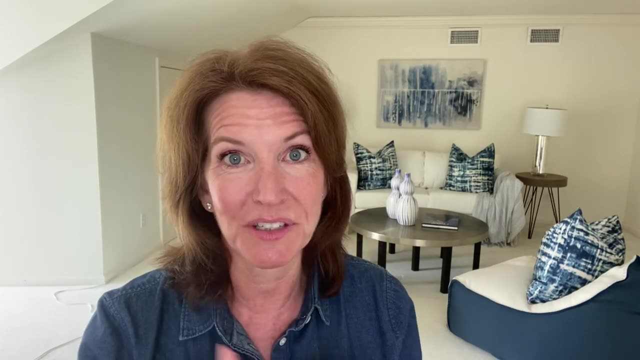 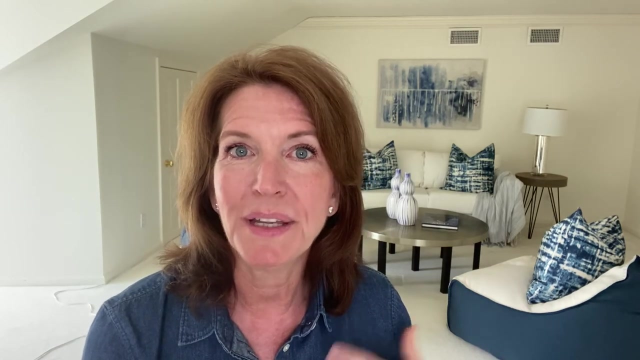 the kitchen helps them develop their fine motor skills and their cognitive skills. So you can, for example, start feeding into what colors are these vegetables? and let's put all the red vegetables over here, and how many carrots can you count there? So there are lots of opportunities when we get. 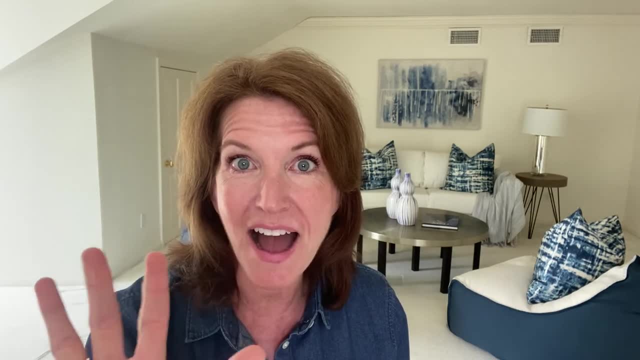 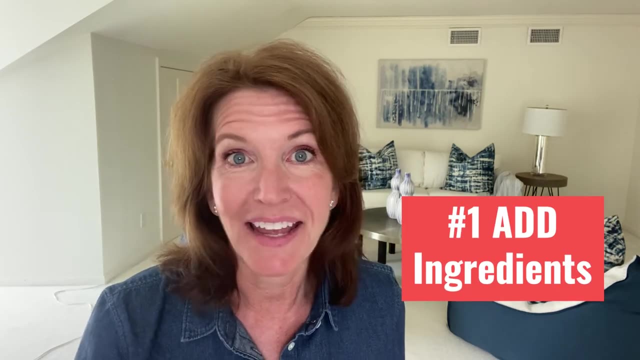 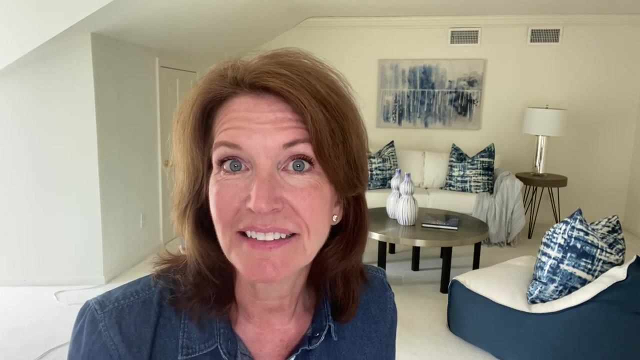 toddlers in the kitchen. So let's talk about those five different ways that toddlers can help you cook in the kitchen. Number one: they can add ingredients from a teaspoon of salt into batter, a cup of flour into batter to tossing in diced carrots. 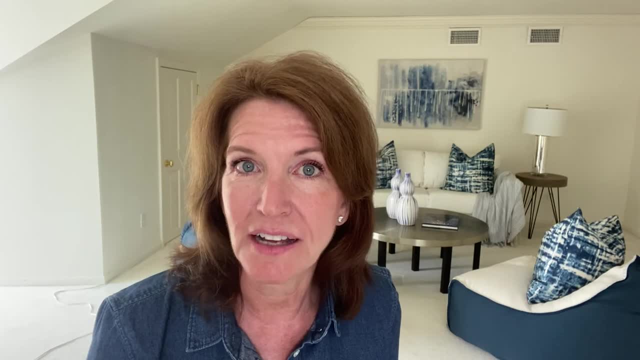 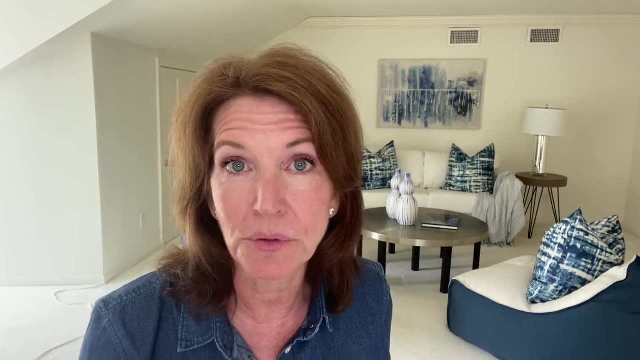 or carrot coins into a salad. let your toddler start to add ingredients to the things that you are making for dinner, for breakfast or for lunch, or even for snack time, Of course, if your toddler's fine motor skills aren't ready to do something like this. 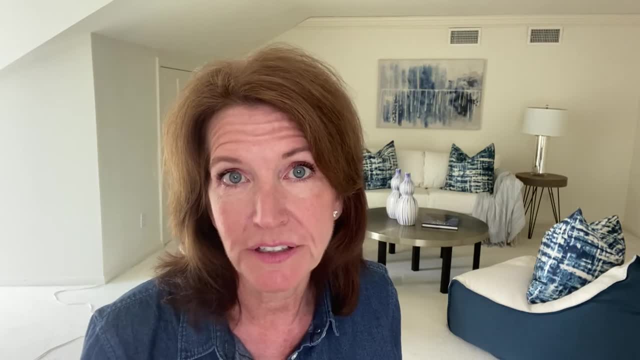 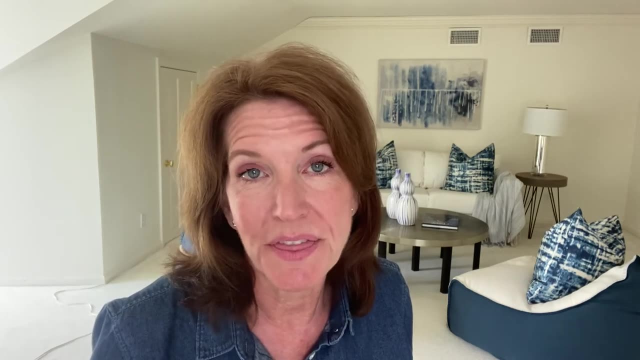 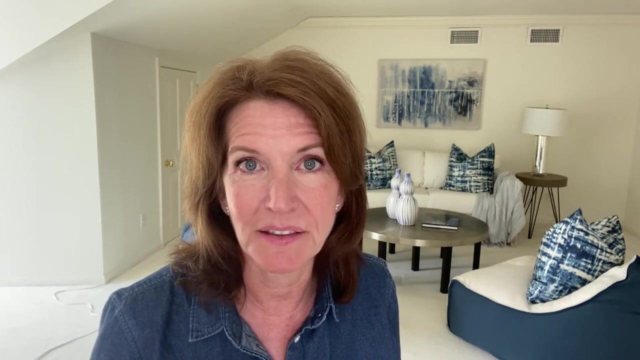 you can help them along. For example, you can fill the cup with flour and let him hold the handle and tip it into the bowl. Starting with that is a great way to get your toddler's fine motor skills up to speed, The more he does pouring and adding. 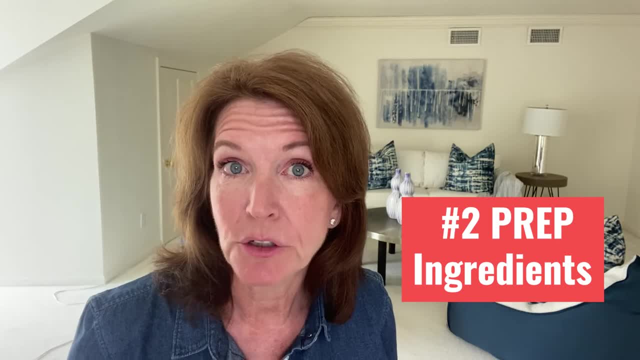 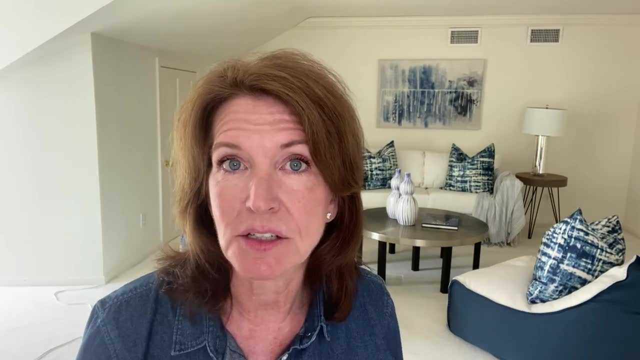 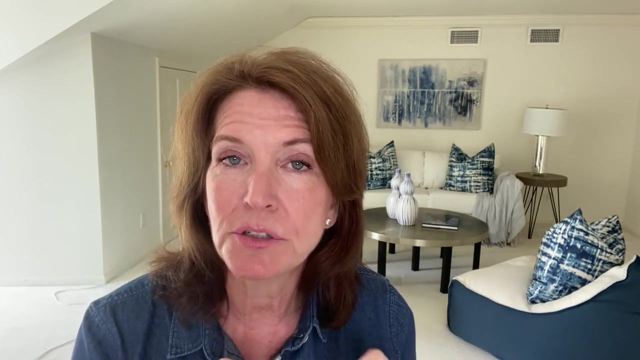 the better he gets at it. Let your toddler help you prep your ingredients. This is the second way that toddlers can get involved. Let your toddler wash produce: washing lettuce, washing fruits, other vegetables. Getting hands on those vegetables helps to get him familiar with vegetables. 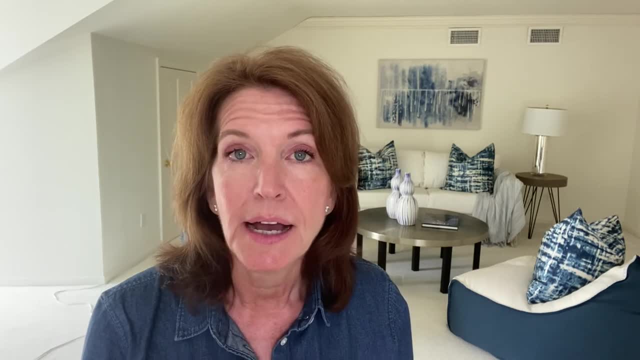 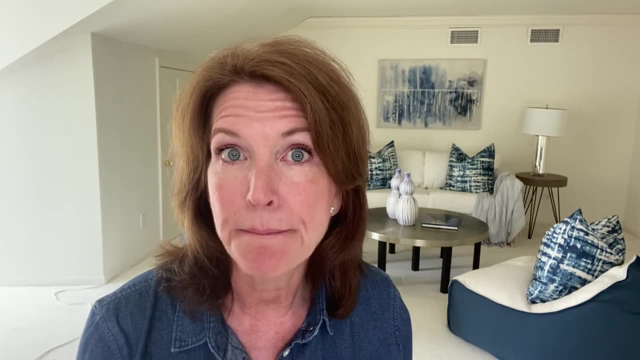 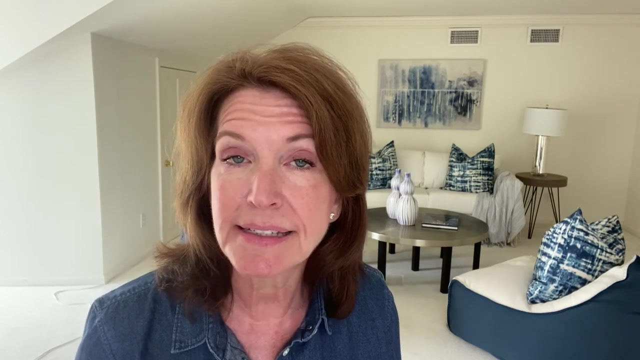 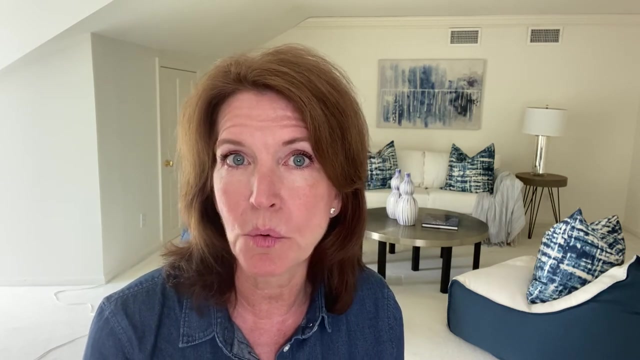 the texture of vegetables and fruits and other foods, which only helps him get informed about what the experience of eating them might be like. This is particularly important for some toddlers who are hesitant to touch things, are maybe a little bit more sensitive to the textures of food or don't like to get their hands. 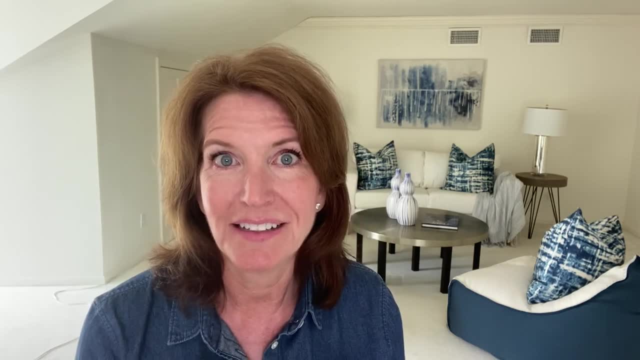 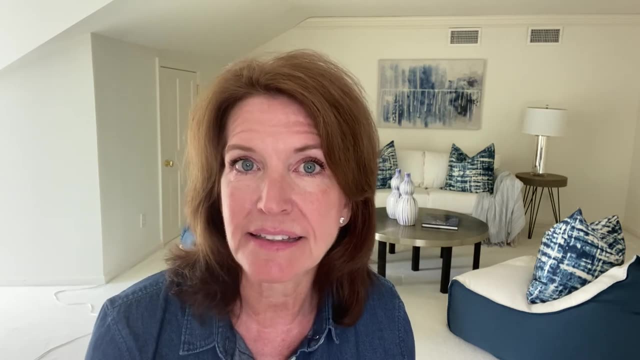 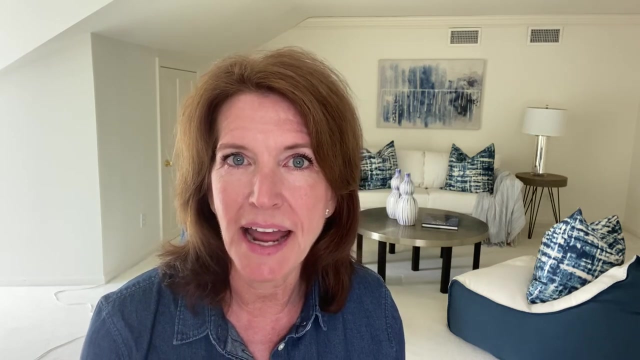 dirty. If you have a toddler like that, it's even more important that you get their hands on food early and often, so you can desensitize those texture sensitivities or other sensory sensitivities that they might have. So for the toddler who doesn't like to get their hands dirty, 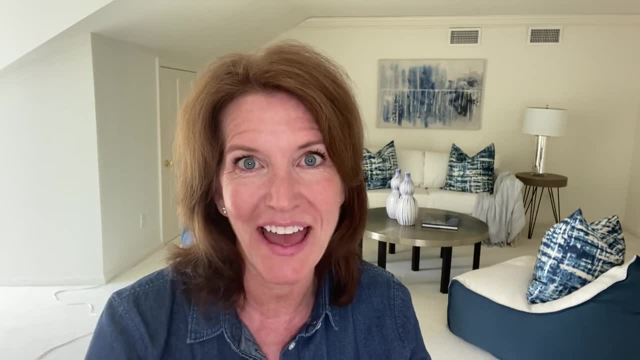 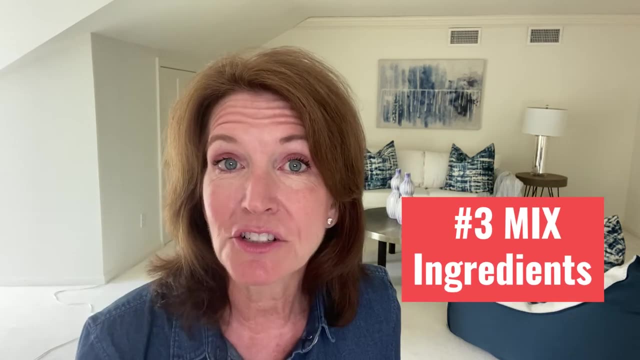 you don't want to avoid those things. You actually want to get their hands into that food and get involved with the food to help desensitize that sensitivity. The third thing toddlers can do is mix. They can mix with a spoon the ingredients. 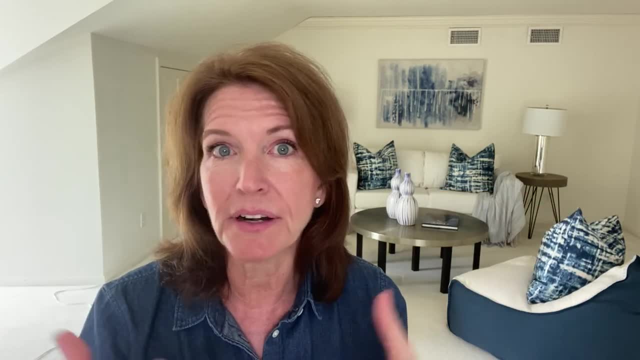 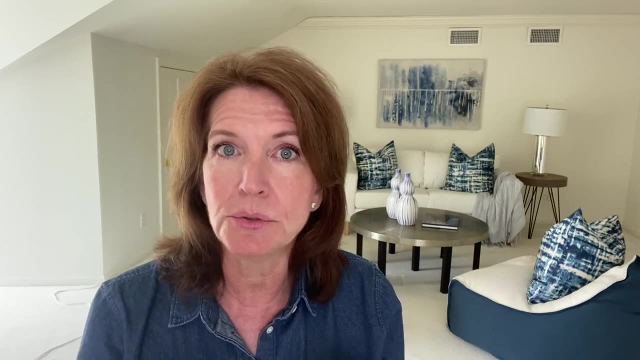 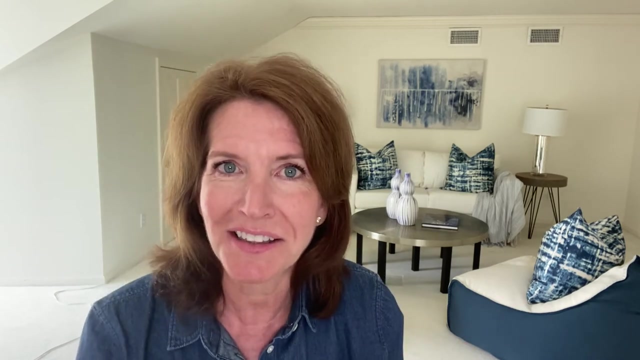 in a bowl. They can mix a salad even with their hands. If their hands are clean. they can kind of mix the ingredients together or, as they get more dexterous, they can use tongs or two salad fork, spoon, salad things- to toss the salad together. If you happen to be a bread maker and you've got 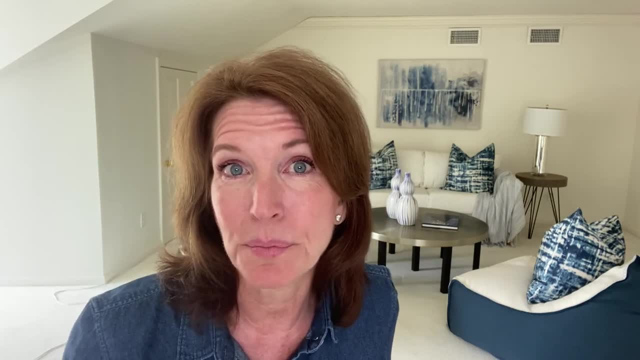 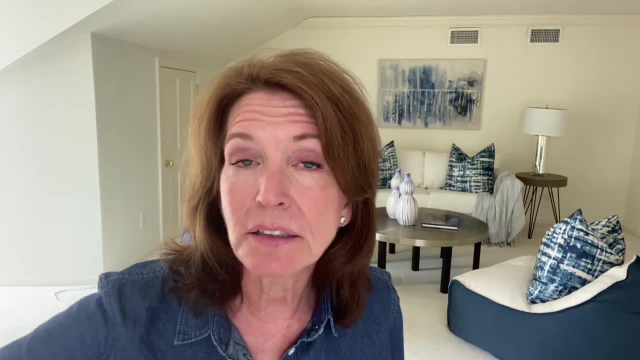 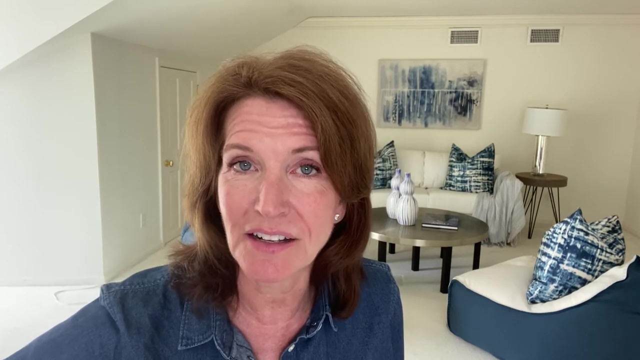 dough of some sort. kneading dough is a great way to help a toddler learn how to mix ingredients together, so it doesn't always have to be stirring. Your toddler can also help you hold a mixer, You holding primarily the mixer, but your toddler having his hand on the mixer can also be a way. 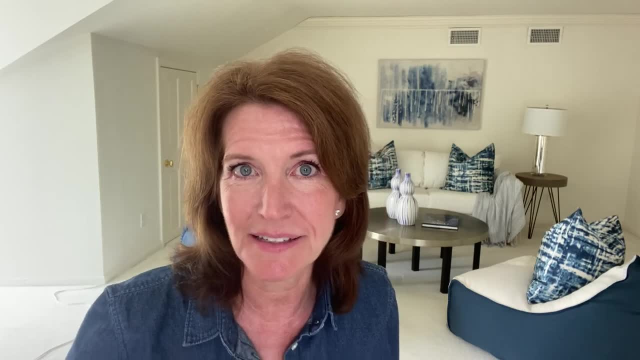 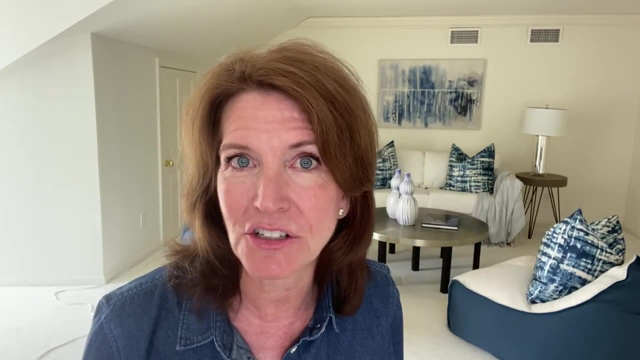 to get him involved in mixing ingredients. Number four is let your toddler gather ingredients and name those ingredients out loud, so your toddler starts to mix the ingredients together. If you happen to be a bread maker and you've got a lot of ingredients in your bowl, you can start to learn the names of different ingredients. 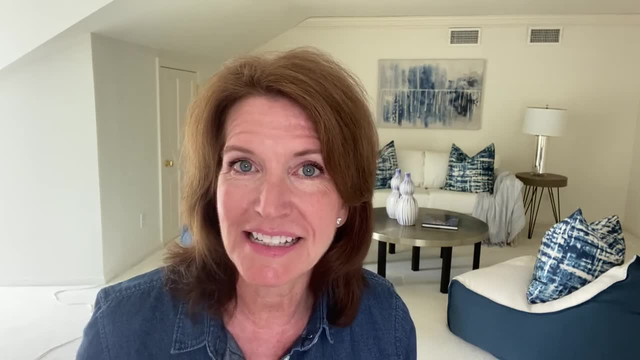 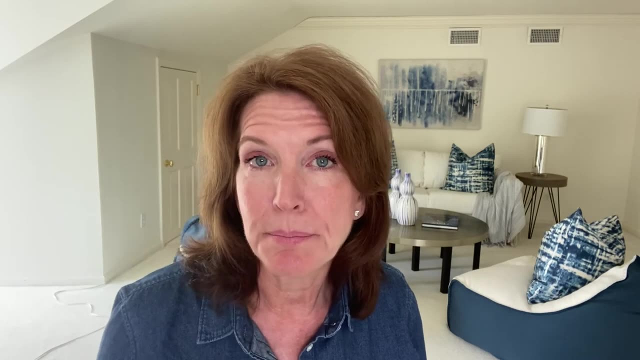 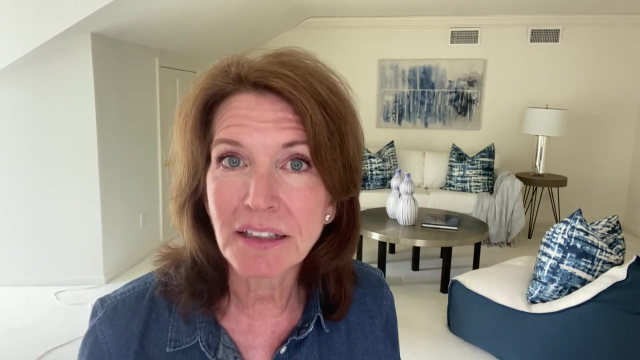 But your toddler can go to the refrigerator and grab a head of lettuce. He can go to the pantry and bring out the container of flour or sugar, or grab a box of baking soda or salt, or grab the bag of chocolate chips, for example. Your toddler can help you gather ingredients. That really is great. 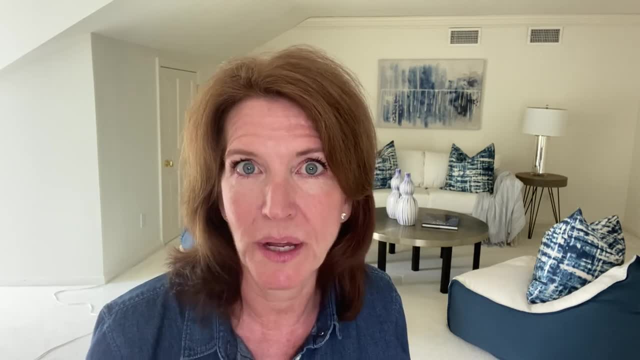 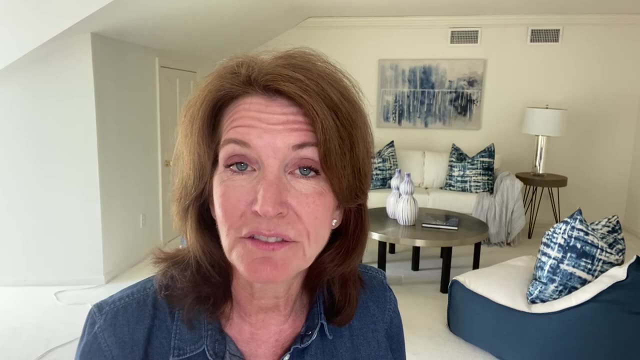 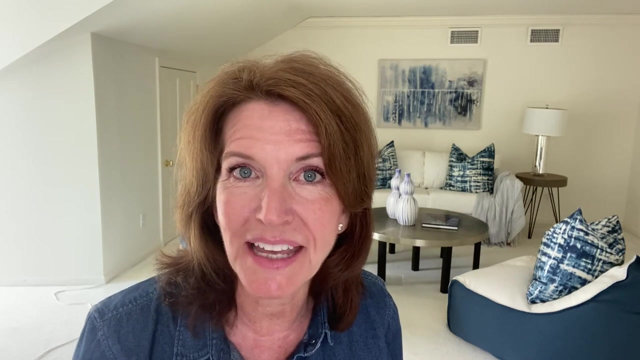 because it gets him involved and he starts to learn what all of those different ingredients are and the names for those ingredients. And then the fifth way you can get a young toddler involved is to get him to clean up with you. You can give your toddler a rag and have him wipe down the 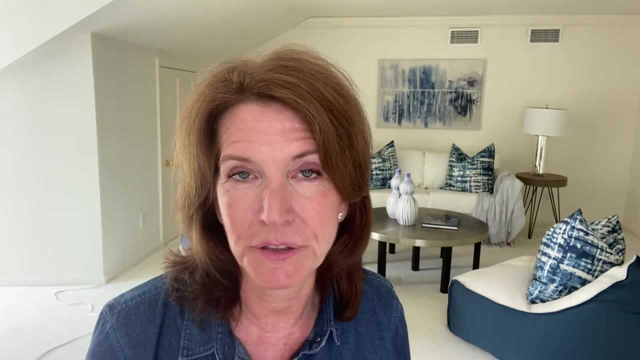 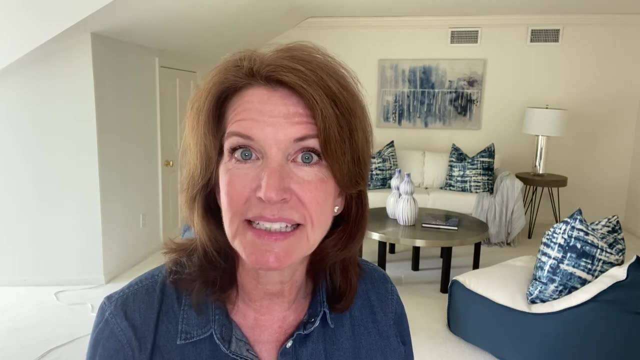 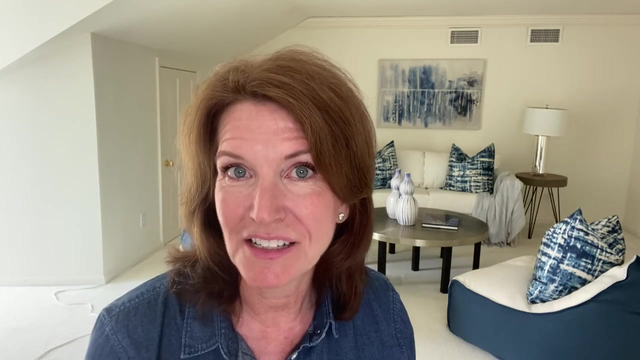 counters before you even get started preparing food. You can have him wash some of the dishes If you have a toddler stool that you can pull up to the sink where he can stand and you can have a dish, a sink full of water and soap. he can wash dishes that are 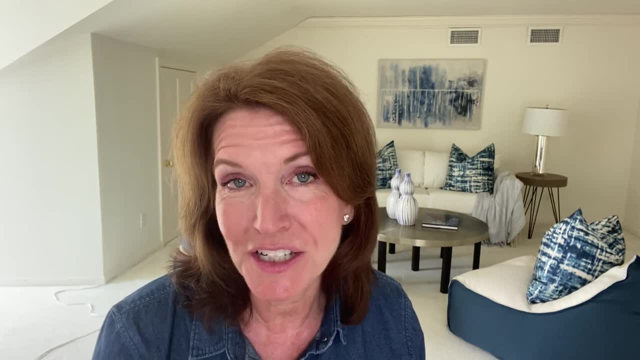 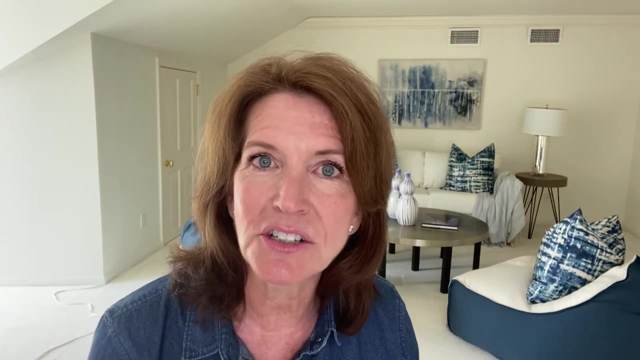 safe to wash, particularly things like measuring spoons and measuring cups that can be made out of plastic. But get your toddler involved in cleaning up so he starts to see the process of cooking, That it's not just sitting down and eating what's made, that there's actually a 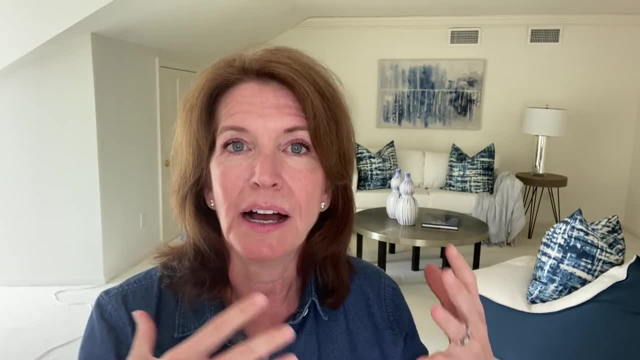 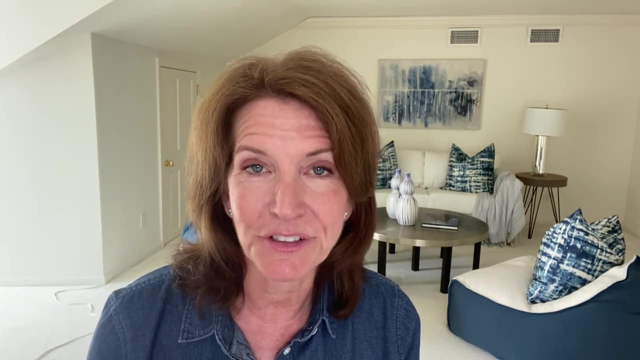 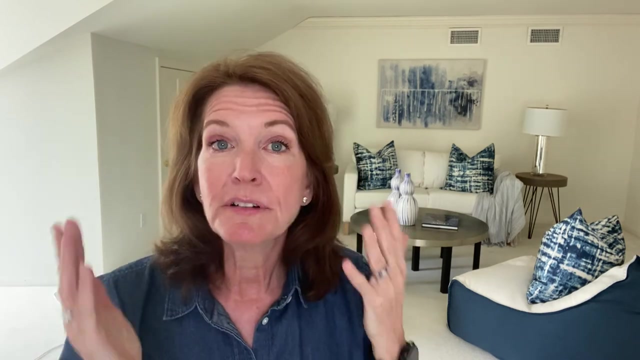 process of cleaning. before you prepare food, There's all the steps involved in actually preparing the food and then the process of cleaning up after food. Lots to learn for toddlers when they are involved in helping you cook in the kitchen. Remember when you're cooking with. 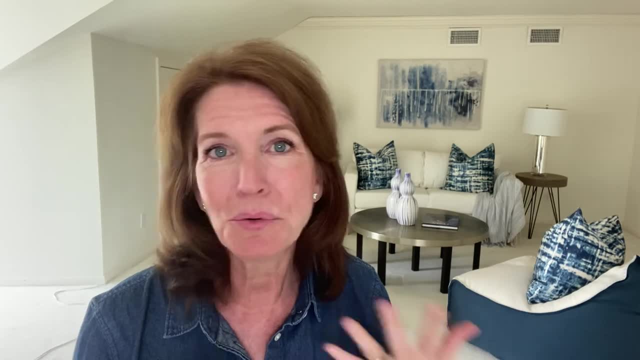 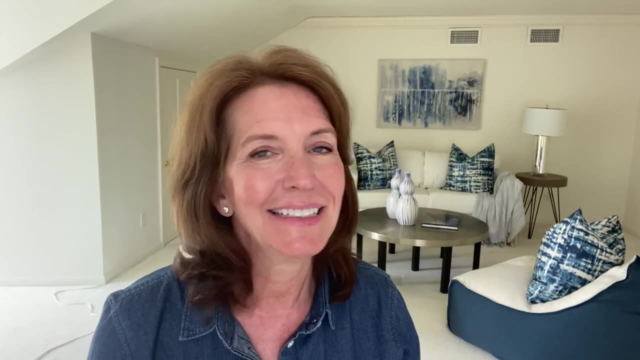 toddlers, you need a great deal of patience. Don't do it when you're in a rush, when you're, you know, coming home from work and you got to get a family meal on the table really fast, That's not a good.